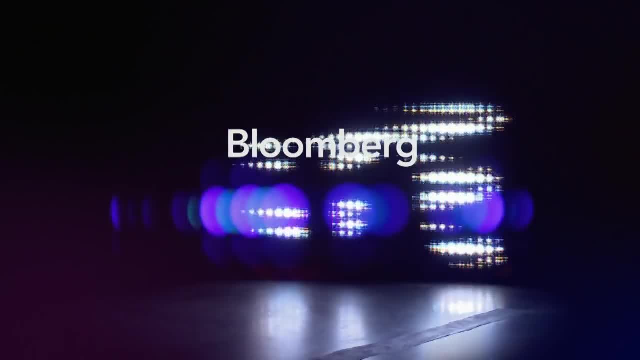 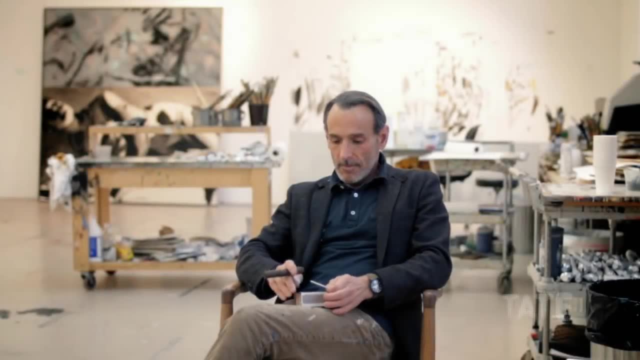 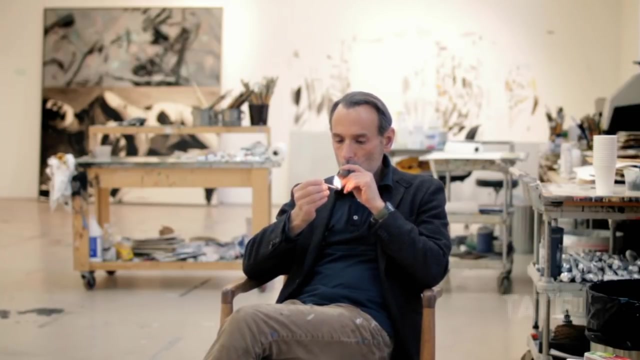 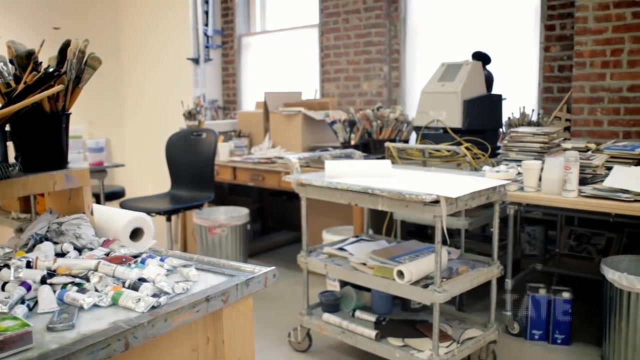 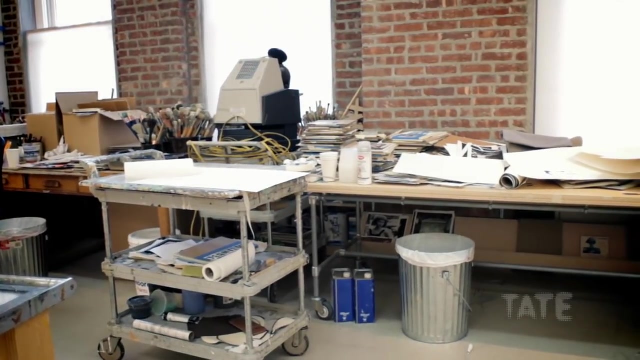 My name is David Salley. We're sitting in my studio in Fort Greene, Brooklyn. I've always been a figurative painter. I was making paintings populated by people in interior spaces when I was a kid And in a way, I've been making the same painting ever since. I 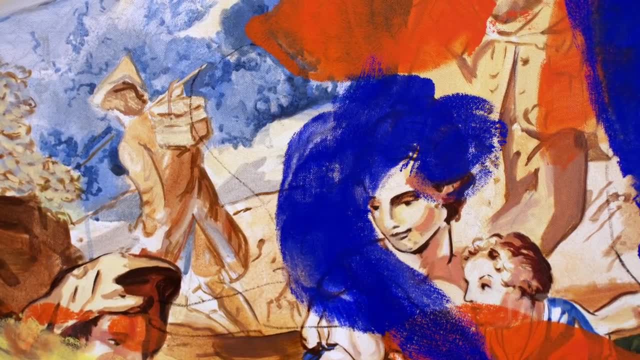 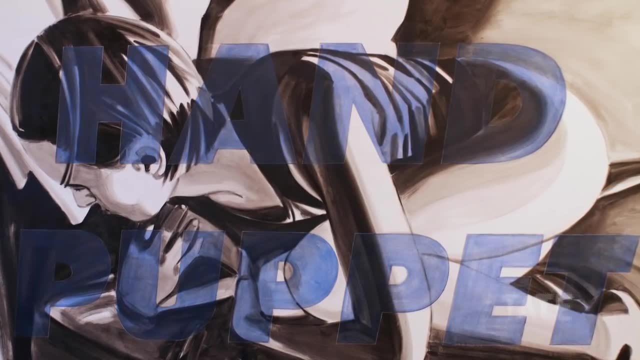 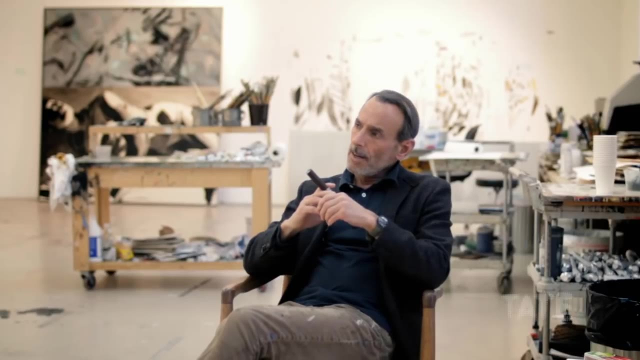 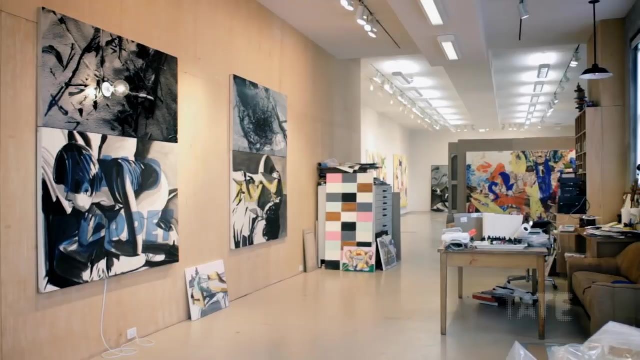 was 14.. When I was younger, I was hungry for a kind of dialogue that centered around intention and meaning And interpretation and things like that. Now I find, as I'm older, I'm just interested in the kind of first level reaction: Yes, no good, not good, finished unfinished. 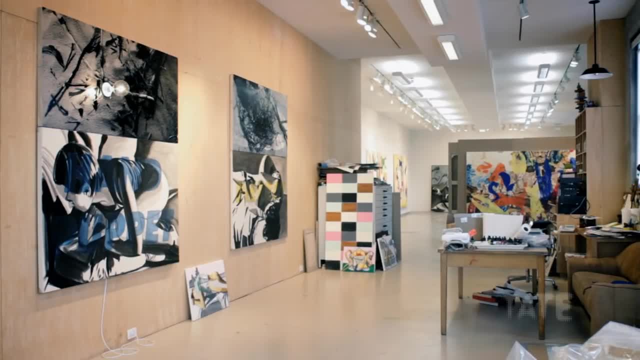 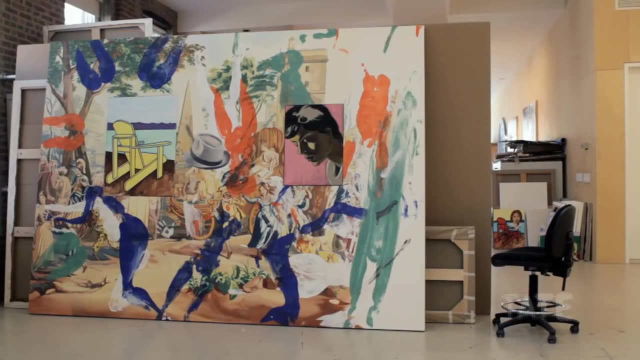 I always start with the complete frame of reference, which is to say the large canvas The paintings are made of. sometimes they're made of a large painting. They have a panel with smaller panels inset into them. I'm not even sure why, but for 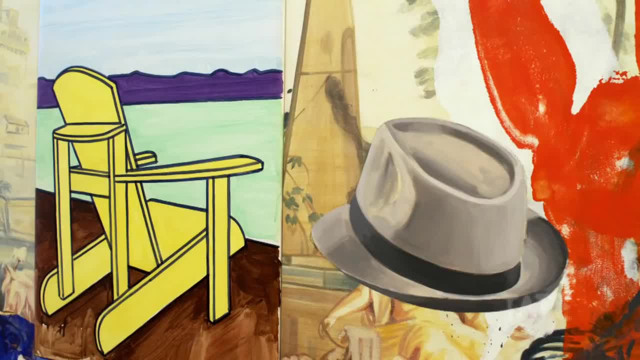 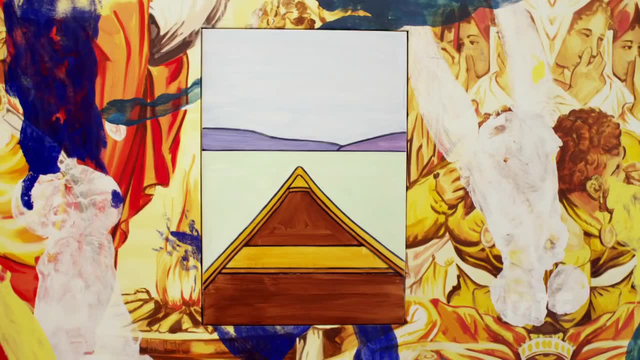 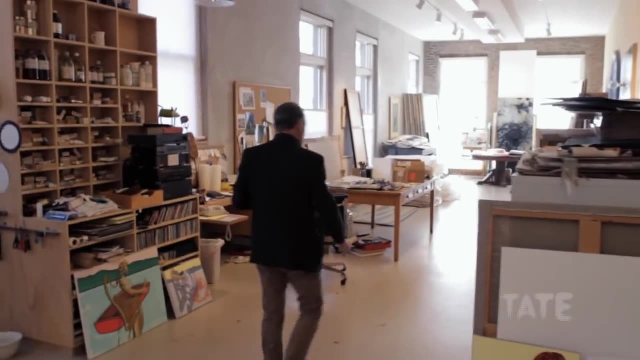 some reason it makes a difference that they're separate panels that are actually set into windows cut in the painting. They're not simply applied on top. The inset panels sometimes function as a punctuation. I don't plan out the works in advance. I have a vocabulary. 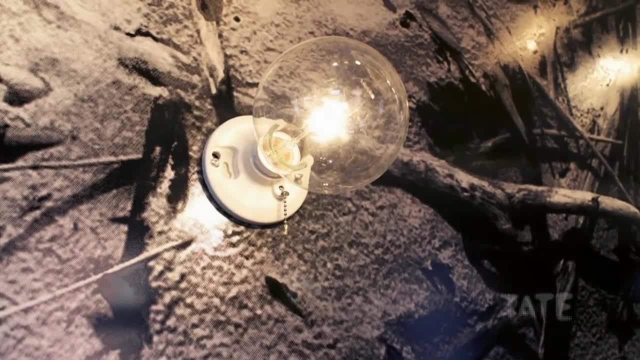 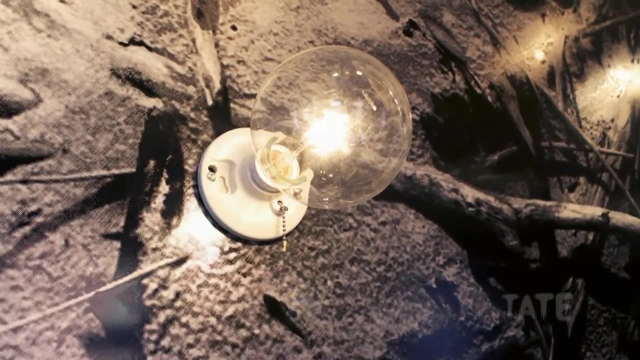 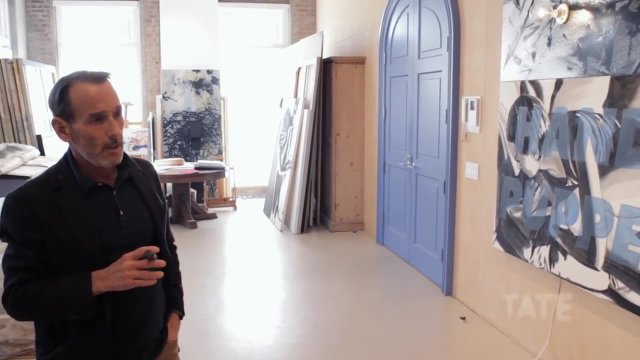 of images and I don't plan out the motifs that I'm working with at any given time in the work, And I know that I want to bring those things into some kind of alignment, but I don't know ahead of time what exactly that alignment's going to be. 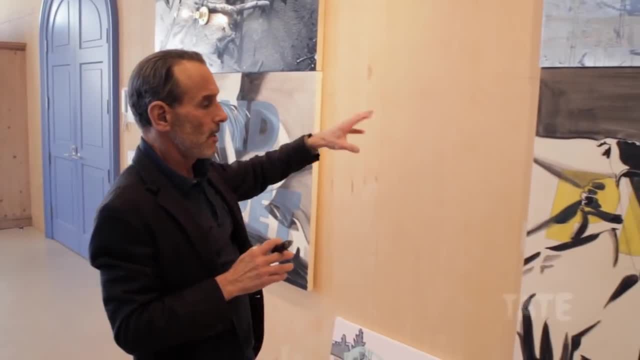 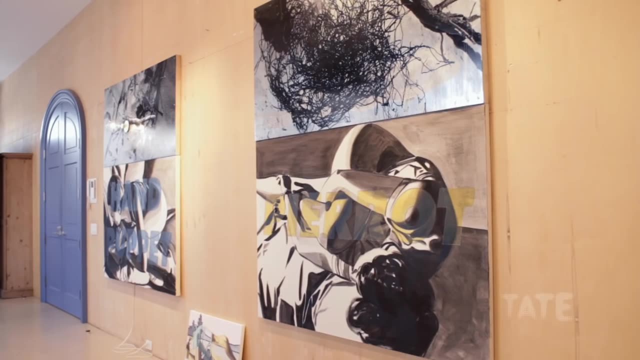 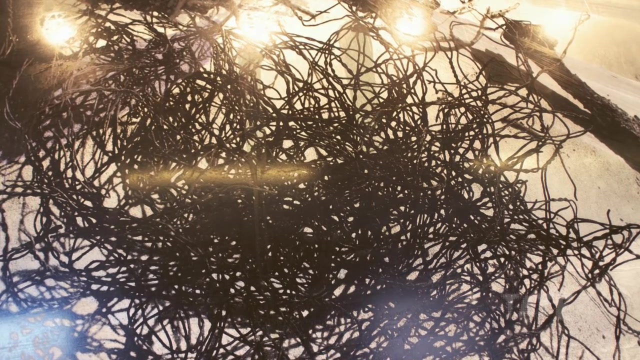 I'm pairing the word or the phrase with a figurative element, a very strongly painted figurative element, and another element which is, in this case, a silk screen made from a photograph I took In this context. I think of it as joining abstraction and figuration.